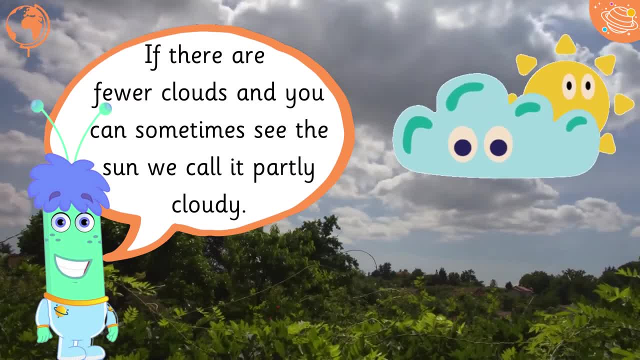 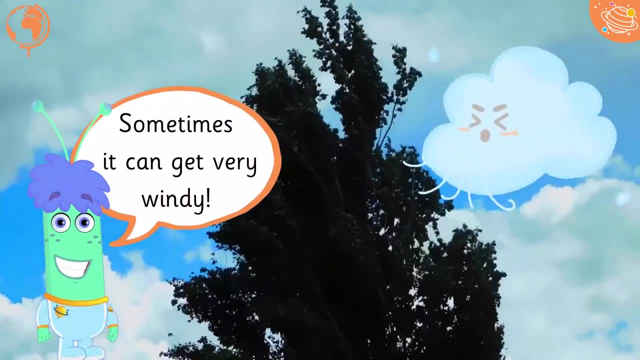 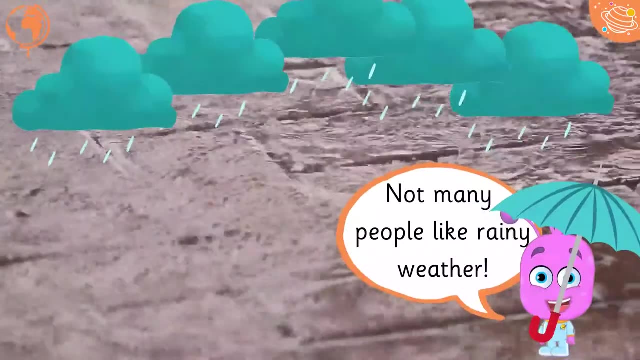 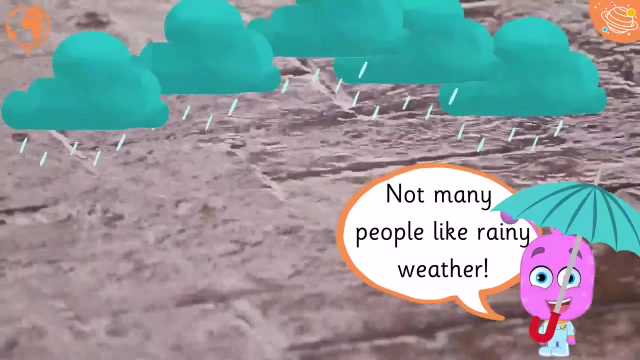 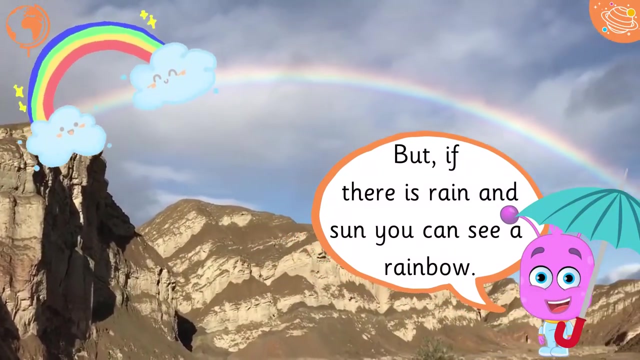 we call it partly cloudy. Sometimes it can get very windy. Not many people like rainy weather, But if there is rain and sun, you can see it. But if there is rain and sun, you can see it. It's like a rainbow. 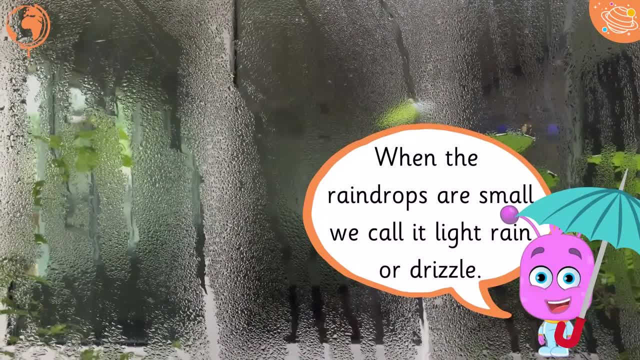 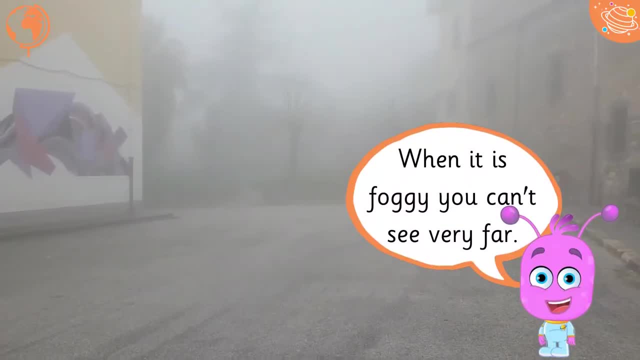 When the raindrops are small, we call it light rain or drizzle. When it is foggy, you can't see very far. When it is foggy, you can't see very far. When it gets cold, we can have snow. 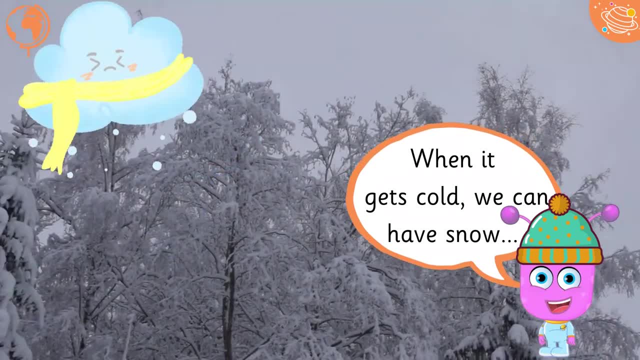 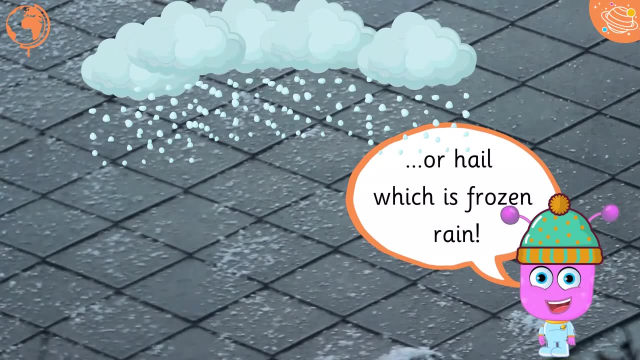 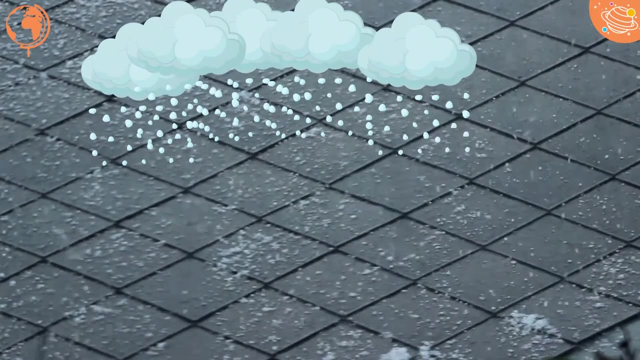 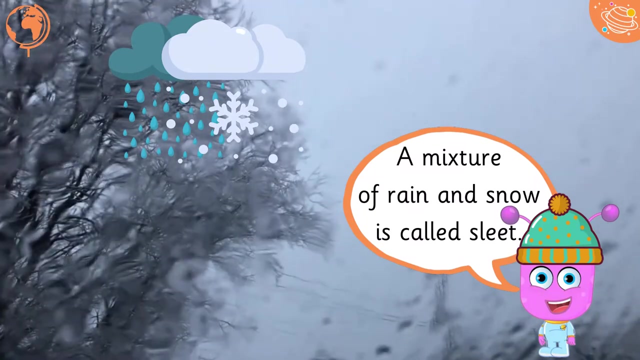 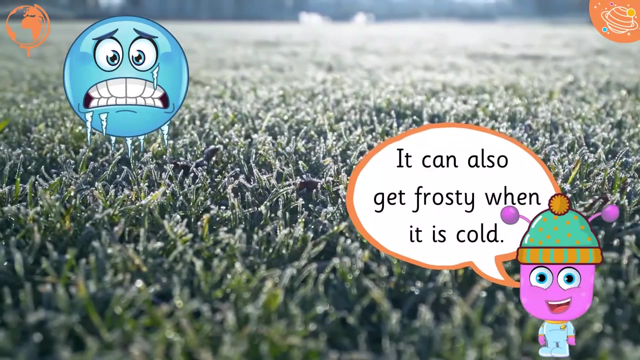 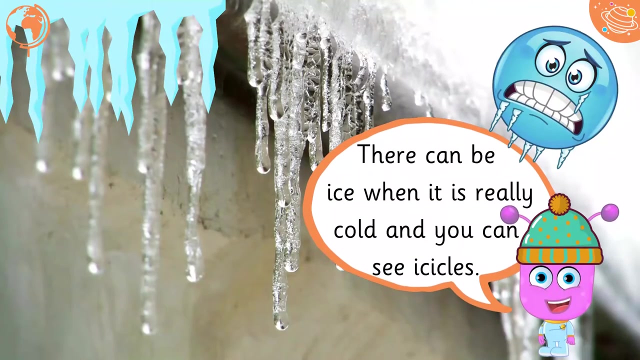 When it gets cold, we can have snow, have snow or hail, which is frozen rain. A mixture of rain and snow is called sleet. It can also get frosty when it is cold. There can be ice when it is really cold and you can see icicles. 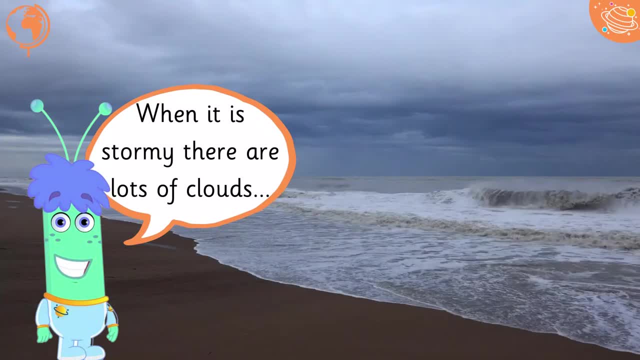 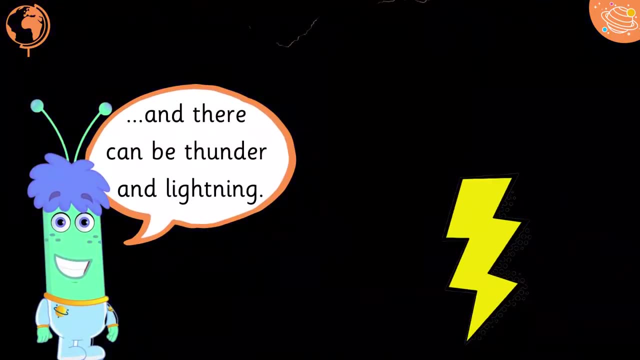 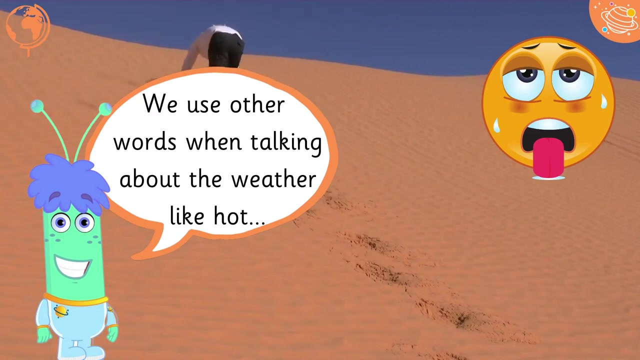 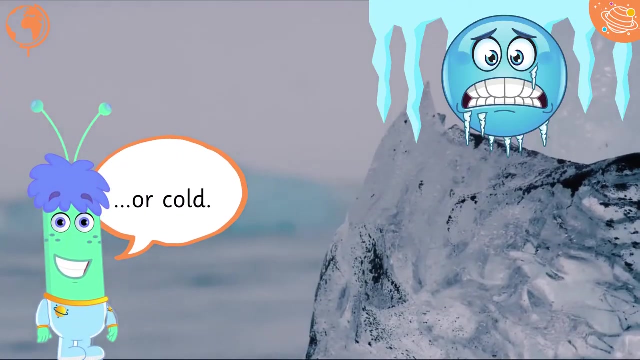 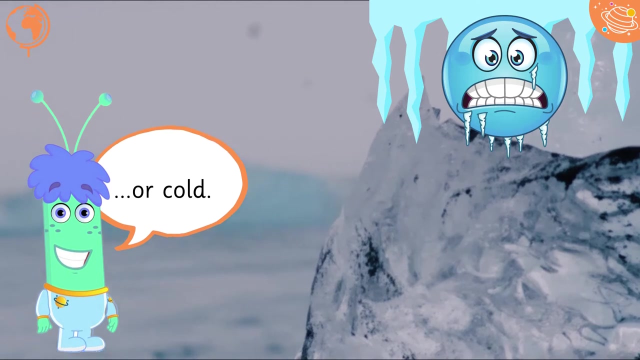 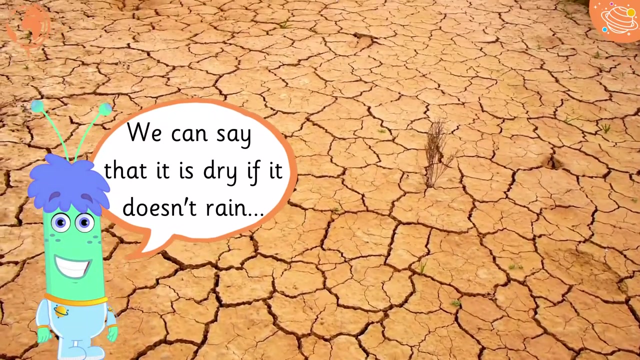 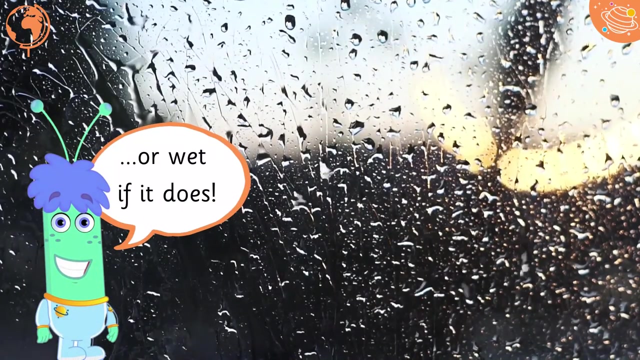 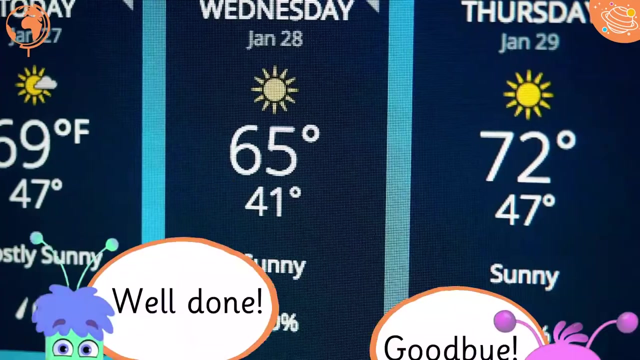 When it is stormy, there are lots of clouds And there can be thunder and lightning. We use other words when talking about the weather, like hot or cold. We can say it is dry if it doesn't rain Or wet if it does.